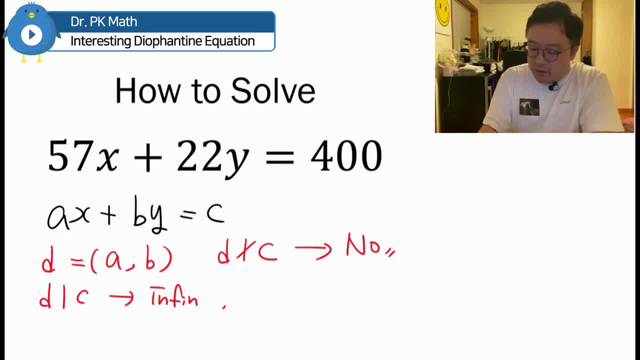 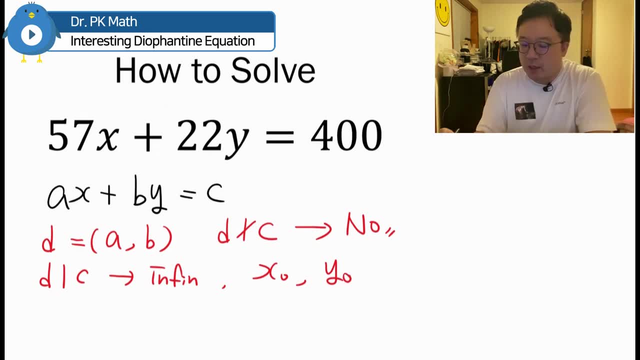 And at the same time, in this case, let me say, x is 0 and y is 0 are two specific solutions for the x and y right, Then we can find, in this case using Euclidean algorithm, Then in this: 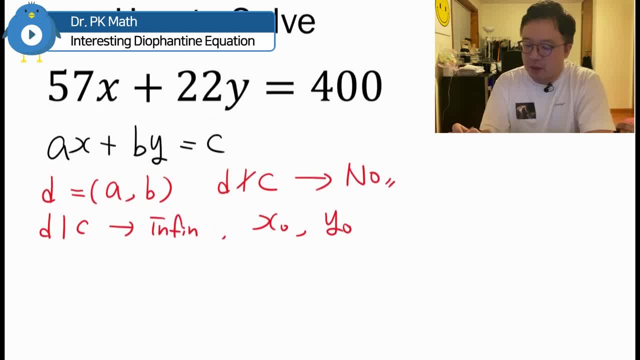 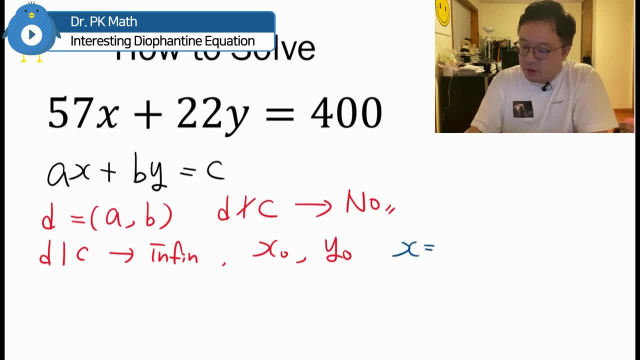 case your x and y. the solution for the x and y in general has to be: x is equal to this, x is 0, and then plus b over d times n, And then your y in general has to be: y is 0 plus minus. 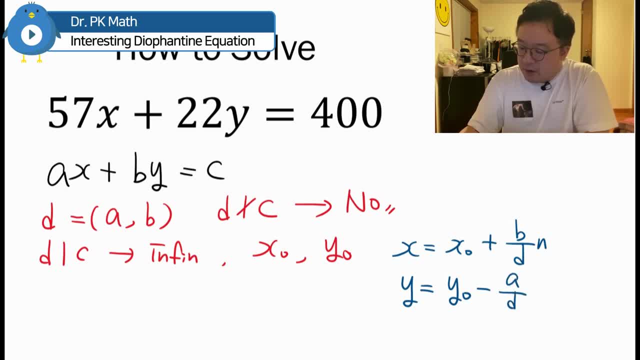 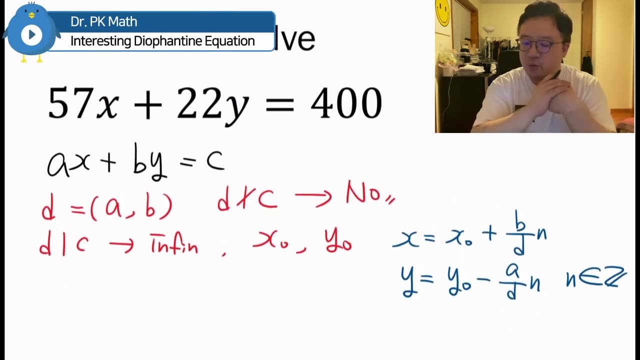 at this time, a over d times n. In this case, n has to be an integer right. We will be using this theorem to talk about this Diophantine equation using Euclidean algorithm right. And So for this case, we have 57 as the A, 22 as B and 400 as C. 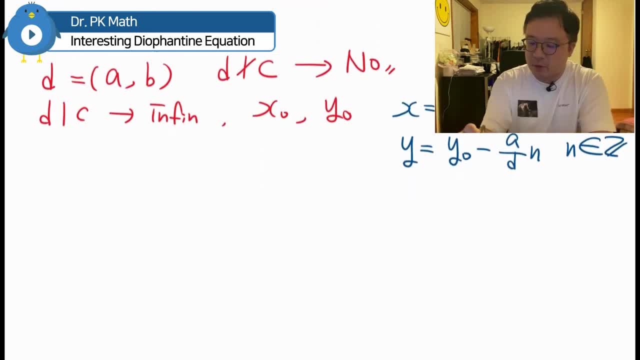 In this case we can find the greatest common divisor of 57 and 22 quite easily, right, You can use repeated division or, in this case, I'll be using Euclidean algorithm to double check, So 57 and 22.. 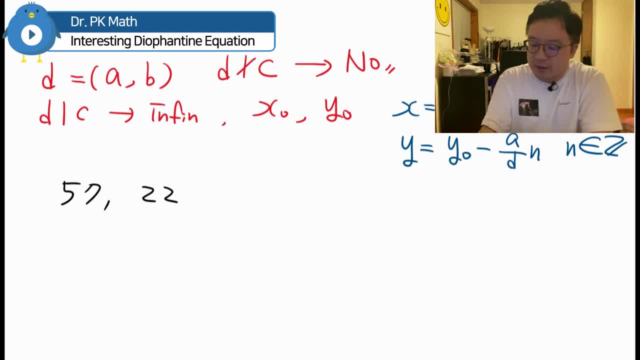 So there's no common factor between these two numbers, except for one right. So that's why we can easily say: your GCD, your greatest common divisor, is equal to 1.. We will be using Euclidean theorem to double check this out, just for the practice right. 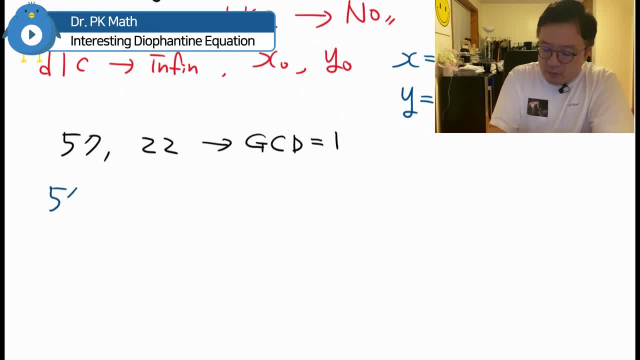 Then 57 is now equal to 22 times 2 plus 13.. Okay, then 13.. Then 22 is equal to 13 times 9 times 1 plus 9.. And then 13 is now equal to 9 times 1 plus 4.. 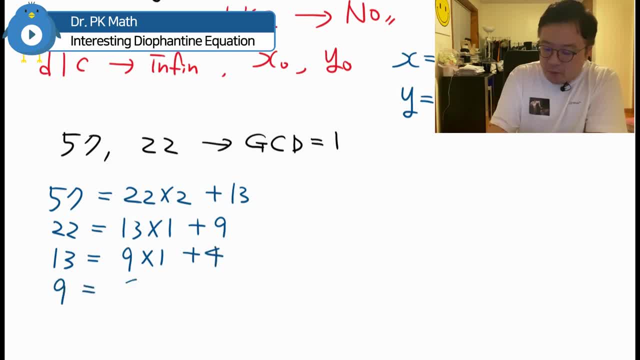 And then 9 is equal to 4 times 2 plus 1.. And lastly, 4 is equal to 1 times 4 plus 0. So this actually makes sure that your GCD has to be just equal to 1.. 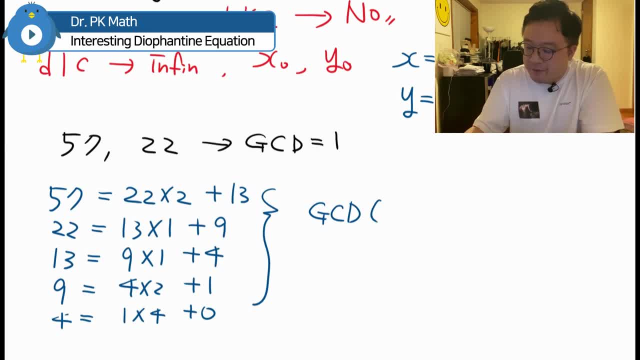 The GCD the greatest common divisor. The GCD the greatest common divisor of 57 and 22.. This is equal to 1, right And at the same time this 1 can divide 400, right. So 1 can divide any number. 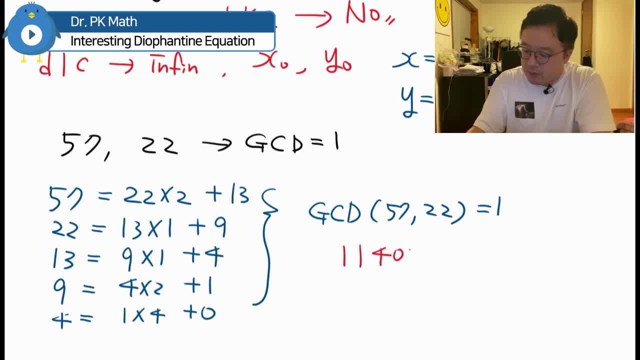 So, technically, 1 divides 400.. So this will actually say that we will have infinite elementary solution. So, in this case, we will talk about now this 1.. So now. So now, at this time, since we double-checked it, 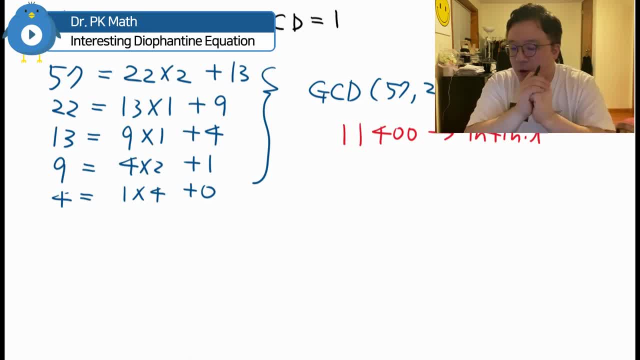 we will have infinitely many solutions for this diaphanin equation. It is all about now getting your X0 and Y0. So one particular solution for X and Y. right After that we can use this nice little theorem to talk about your X and Y solution in general. 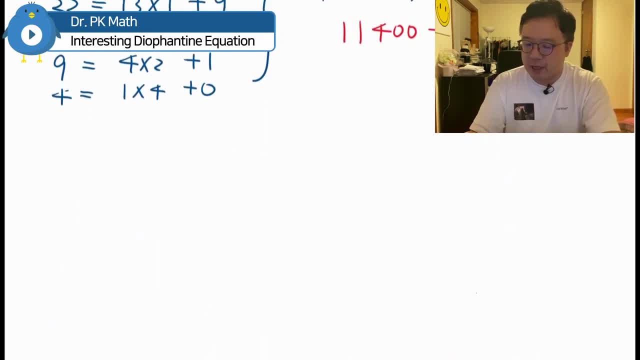 So now we will be getting actually X0 and Y0.. Now let's go back and talk about this number 1, which is your greatest common divisor. So we will be using actually numbers backwards From this Euclidean algorithm. 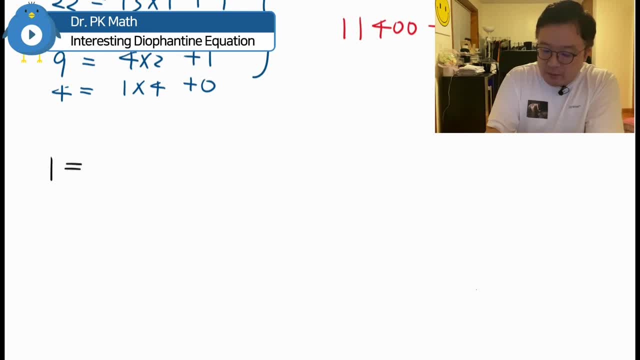 So 1 is now equal to 9 minus 4 times 2.. So we will be using those numbers that we used in Euclidean algorithm backwards right. So now, at this time, this is equal to now 9,. 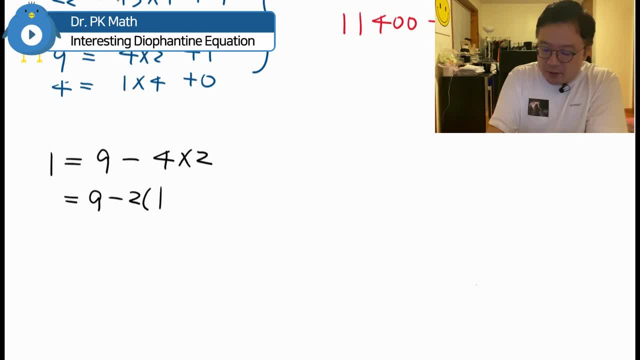 and then minus 2 times 13, minus 9.. Using those numbers as much as possible, then this is equal to 3 times 9.. Minus 2 times 13,. right, And we can rewrite this as 3 times parenthesis, 22 minus 13.. 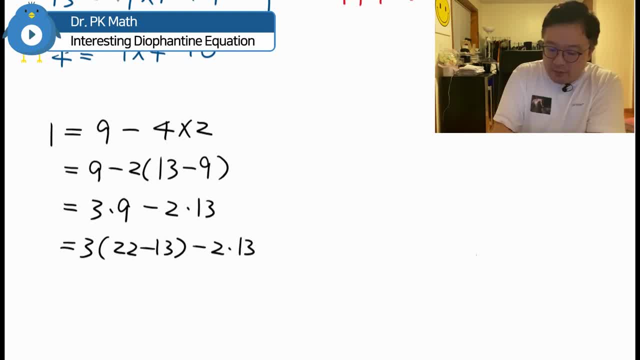 Minus 2 times 13.. Now, at this time, it is 3 times now 22.. This is equal to 3 times 22 and minus 5 times 13.. Right, Then we can- actually we can actually work on this. 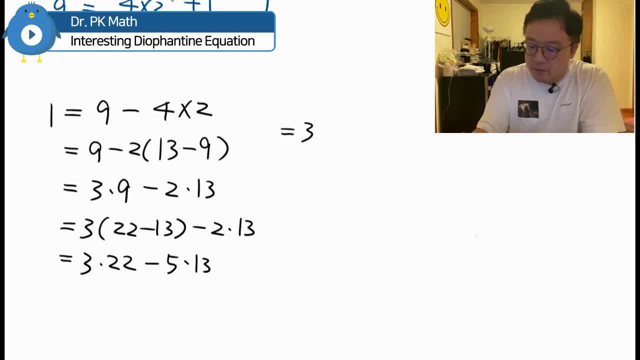 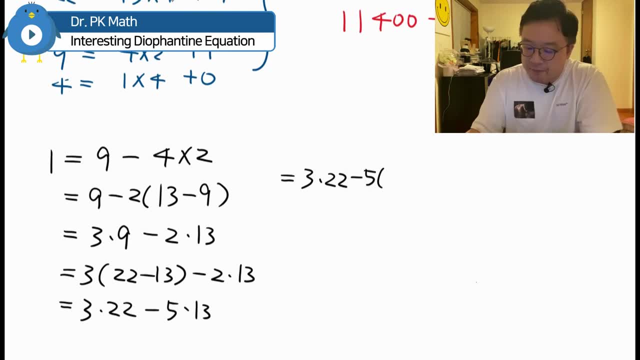 We can actually keep going on. This is then going to be equal to 3 times 22 minus 5- parenthesis- 57 minus 2 times 22.. Right, Then, this is going to be then equal to, using this number: this is equal to 13 times 22 minus 5 times 57..